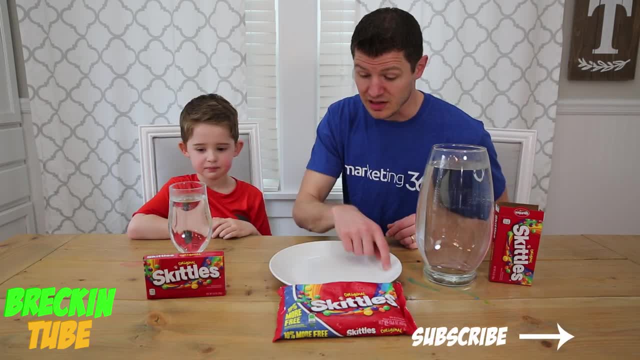 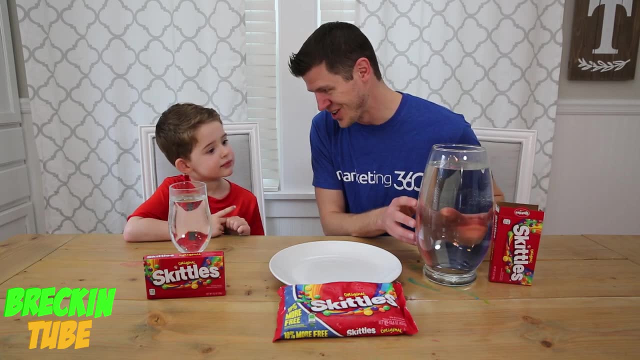 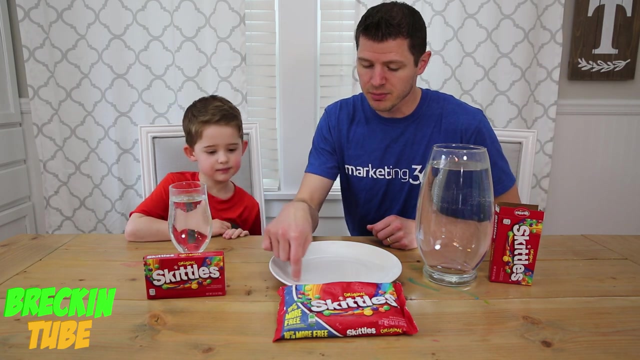 Yes, You need some warm water and then a plate. We also, if you stay to the end, we have a very exciting rainbow waterfall skills experiment to show you, So make sure to stick around to the end. So this is an easy one. All we're going to do is we're going to open up the Skittles. 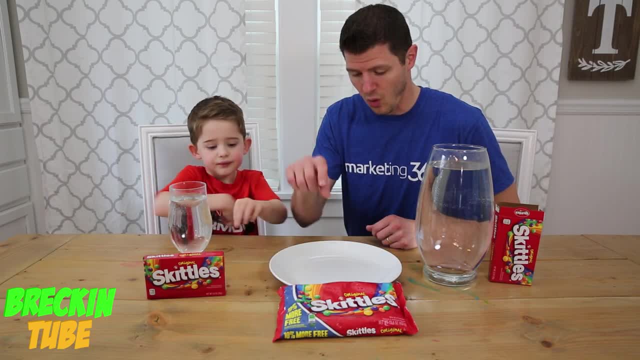 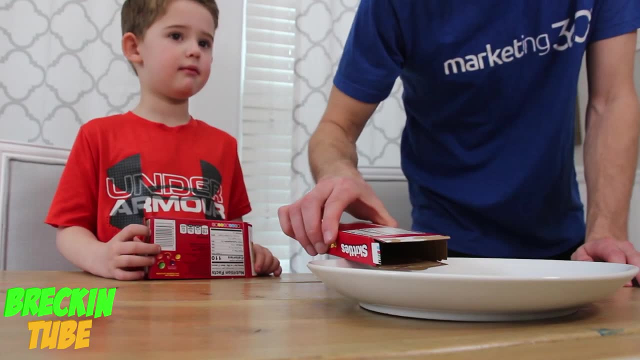 place them all around the edge of the plate, and then we're going to put warm water in the middle. So let's get started. First step: we're going to put some Skittles on to the plate, And then what we're going to do is you're going to want to put these in a rainbow. 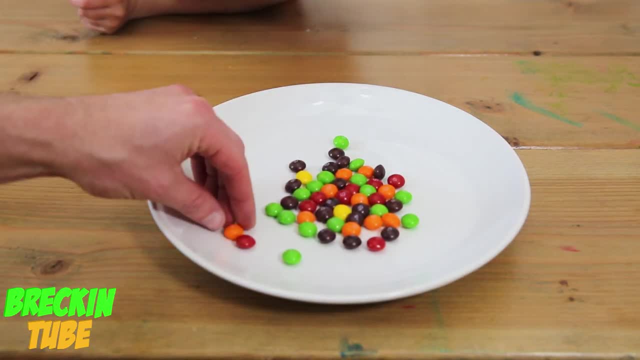 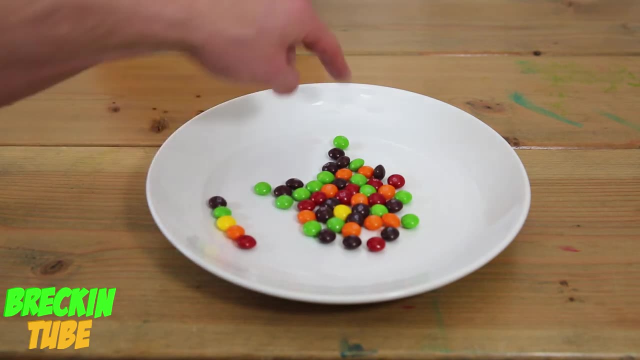 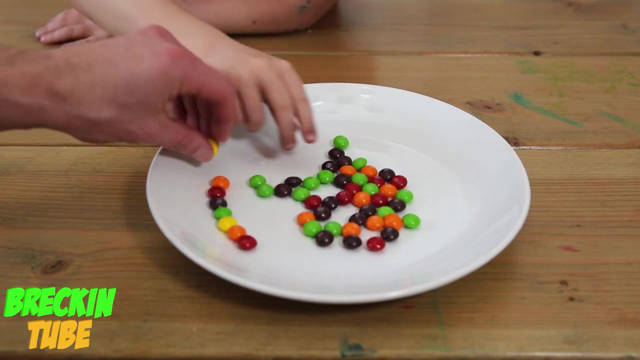 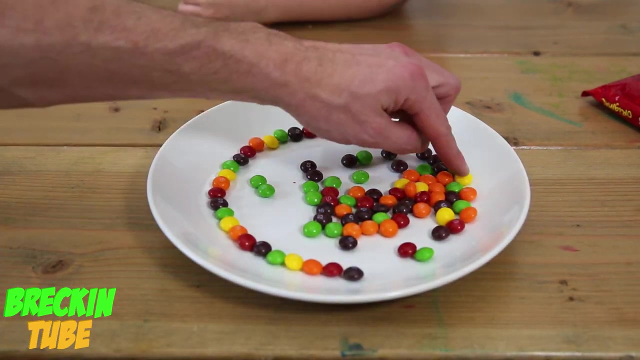 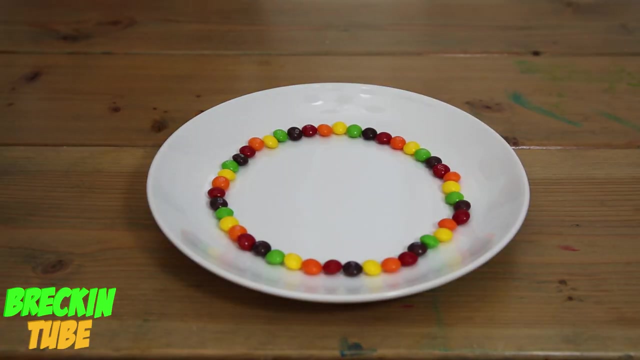 So let's do red orange, yellow, green and then purple. So can we do that all around the edge: Red orange, yellow. Okay, so now what we're going to do Breckin, Breckin is we are going to pour in this warm water into the center. 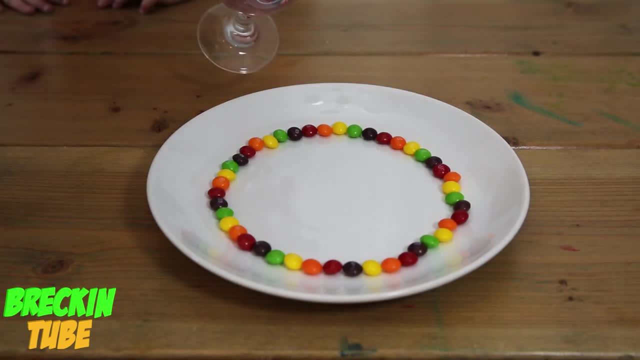 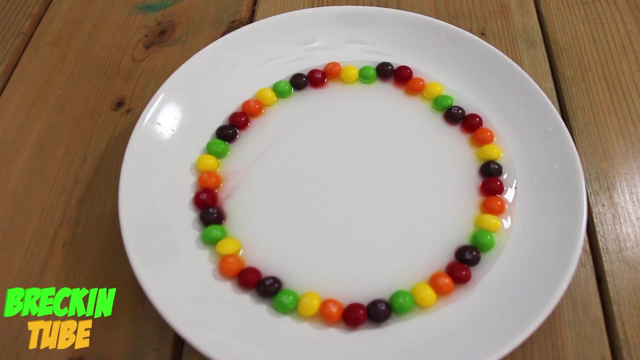 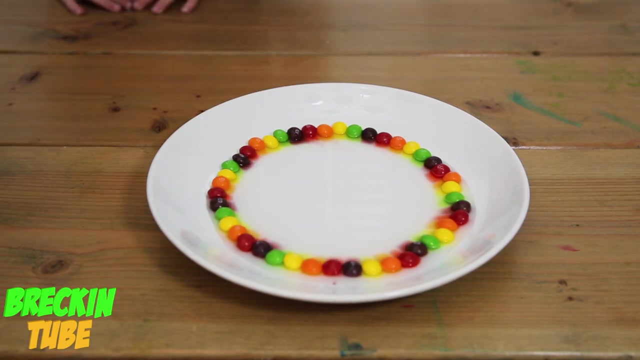 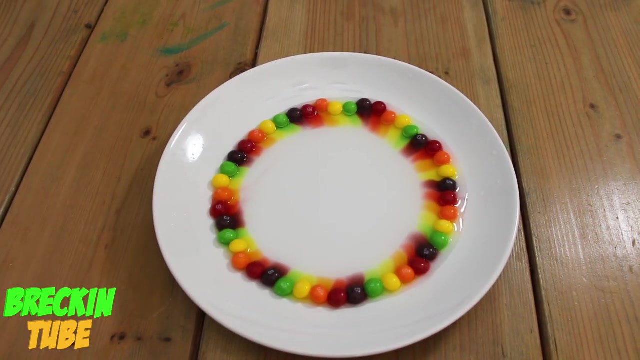 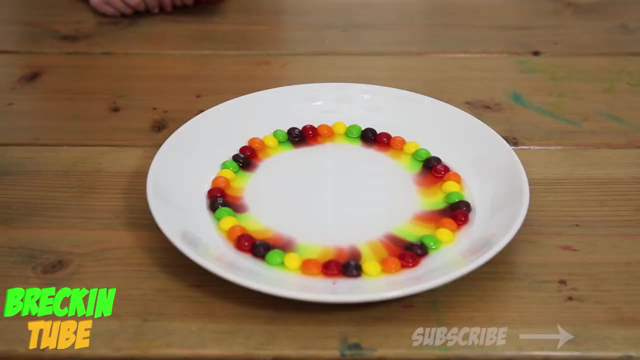 And let's see what happens. You ready? Nothing, Nothing happened, Nothing's happening. Oh my goodness Breckin, what's it doing? Wait, Oh my goodness Breckin, what's it doing? What do you think, buddy? 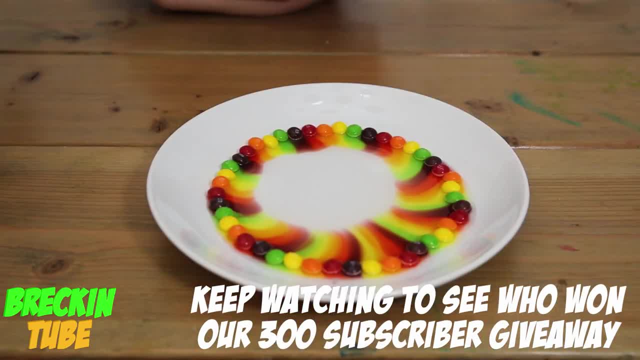 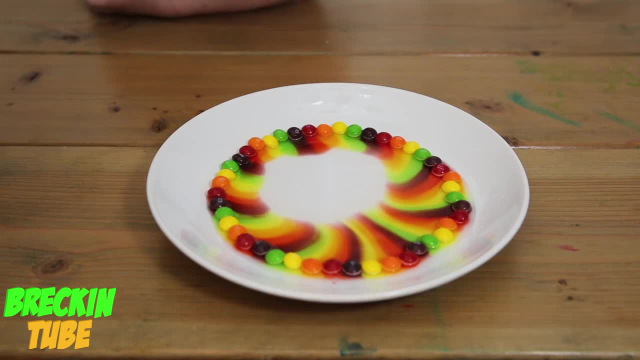 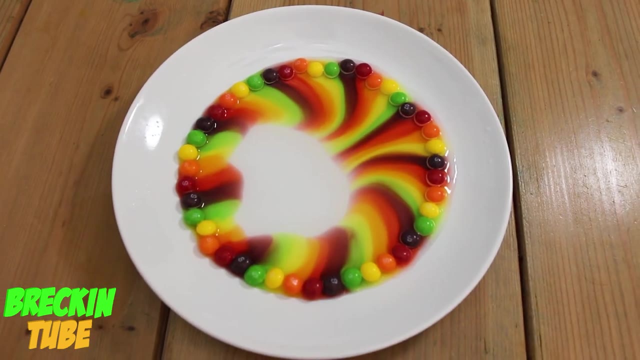 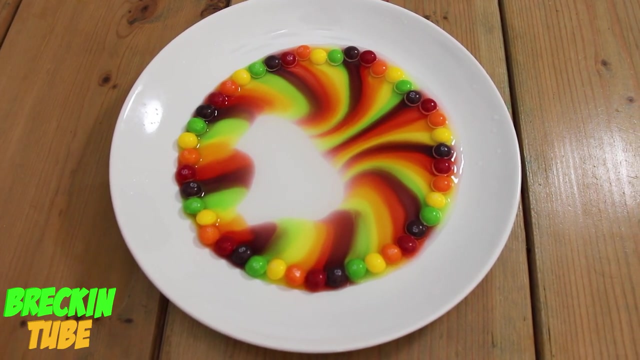 What do you think, buddy? Wow, It is making a cool swirl, isn't it? Wow, That is so neat. How is it doing that? Oh no, I think all of the sugar is getting pulled off by the warm water. 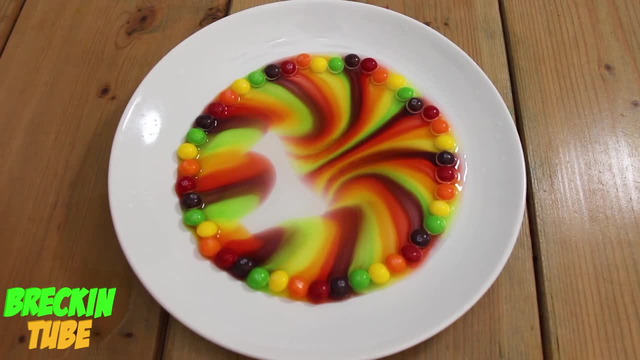 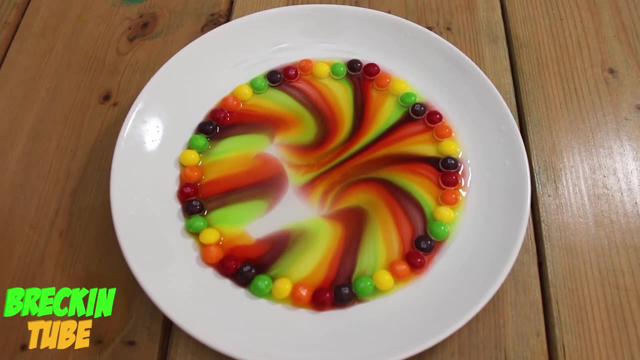 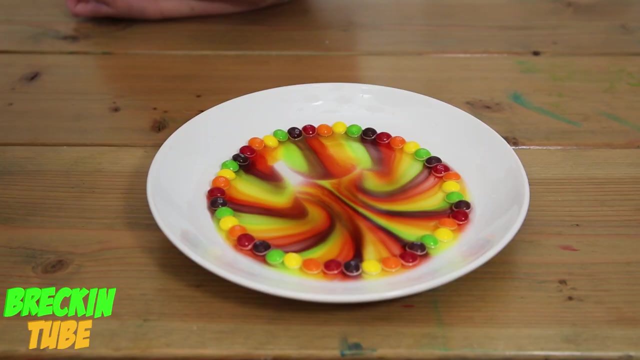 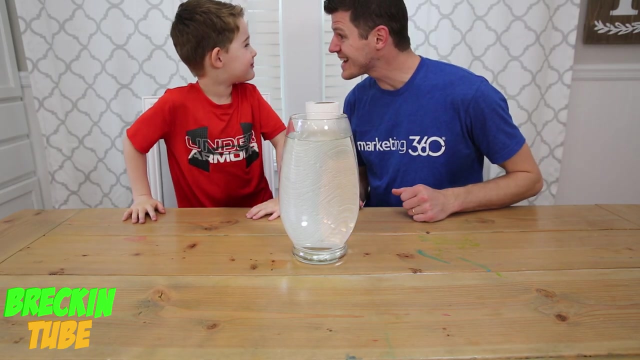 That's a really neat design, isn't it? Wow, So neat. Is it touching? Wow, Is it all covered? Oh, wow, That is super cool, Breckin, Okay, Breckin. what did you think of that experiment? 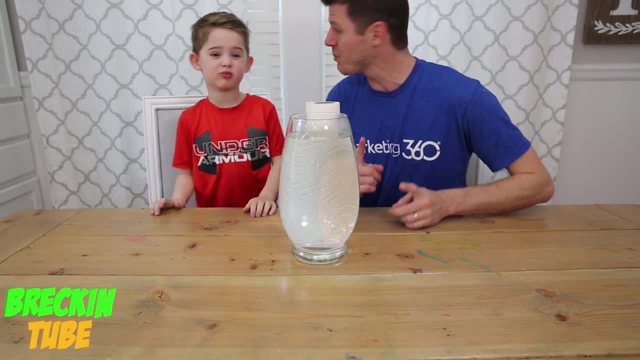 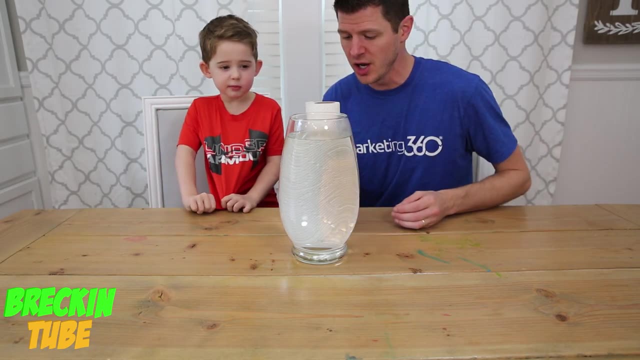 Was that super cool? Okay, guys. So now we have one more Skittles experiment. We're going to try and make a waterfall rainbow. So we have this giant glass of water. We've taken this white paper towel and we just stuck it right. 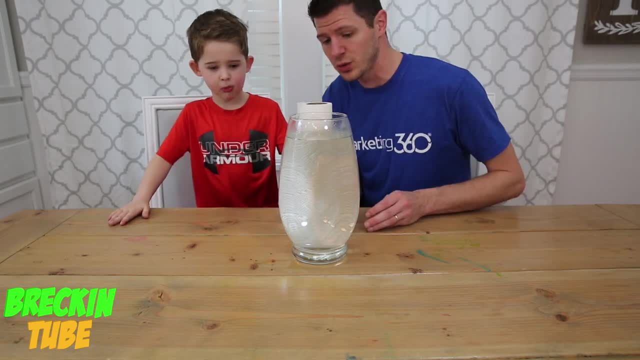 Right behind here, because we're going to try and make sure you can see all of the white through here. Okay, so we're going to put that right there behind it. Now we're going to take these Skittles and we're going to dip them in and see what happens. 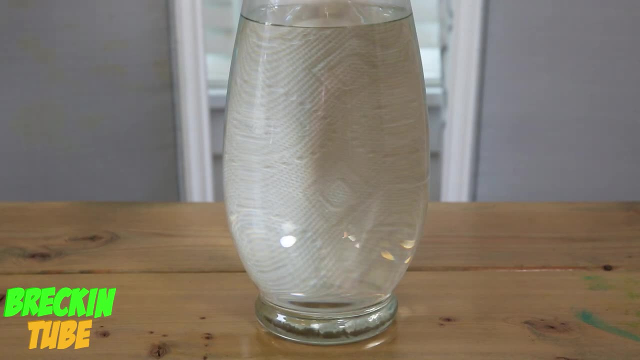 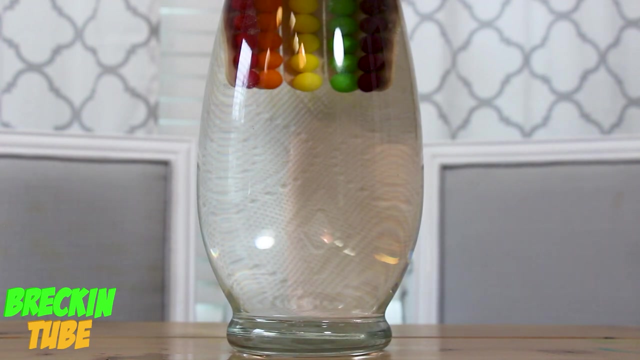 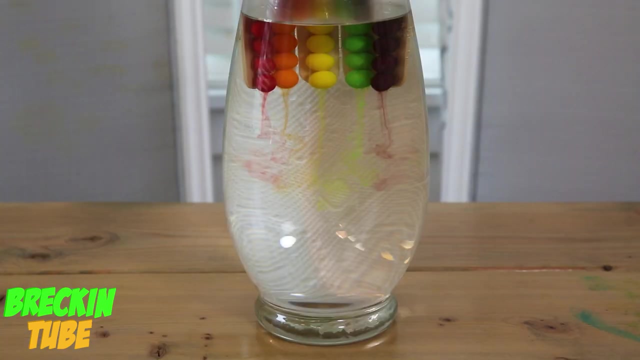 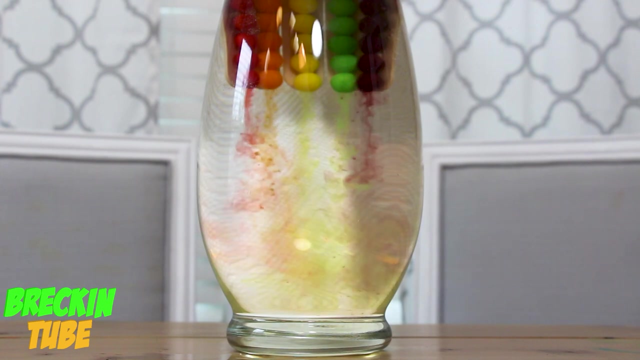 We're going to put these inside there. One, two, three go. How is it happening? Let's see if anything happens. Do you see? Do you see that? Yes, Oh, man Breckin, what do you think? 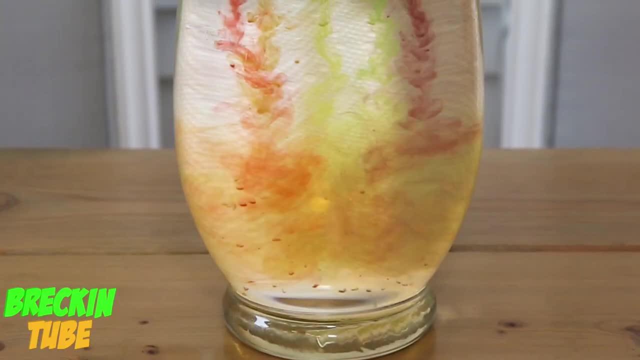 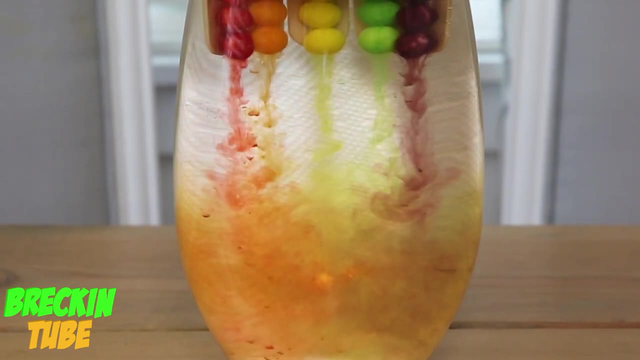 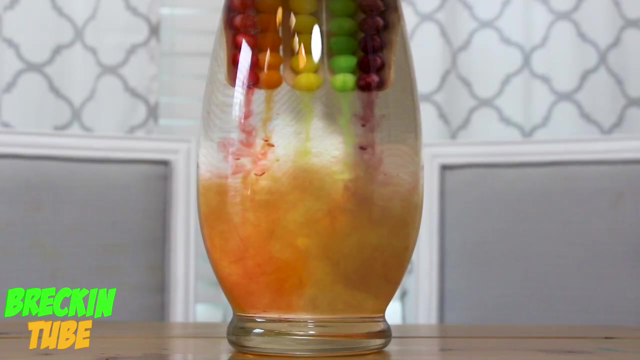 I need to go in the back and see this. What in the world is happening, What is going on? Wow, that is so cool. This is so awesome. Wow, Breckin, that was awesome. Did you see that waterfall? 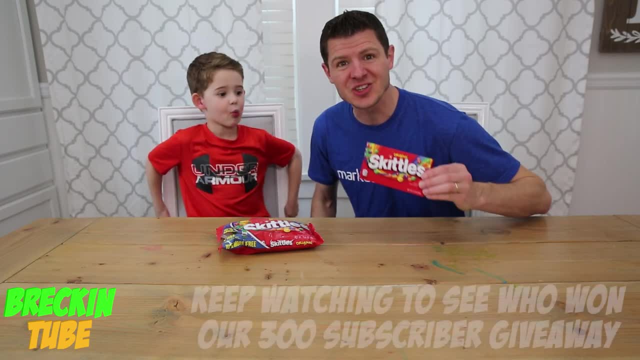 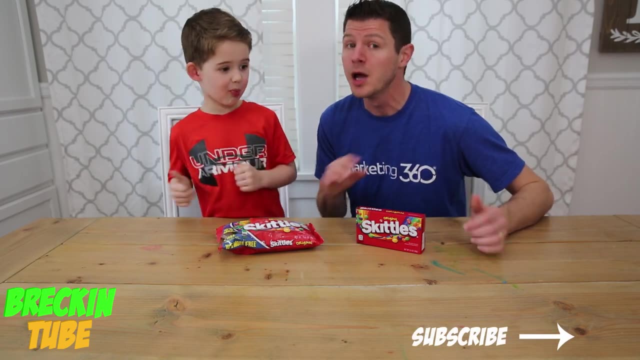 That was so cool. Hope you guys liked that at home. That was our Skittles science experiment. Thank you very much for watching. If you enjoyed the show, don't forget to hit that subscribe button. Please like it and leave a comment. 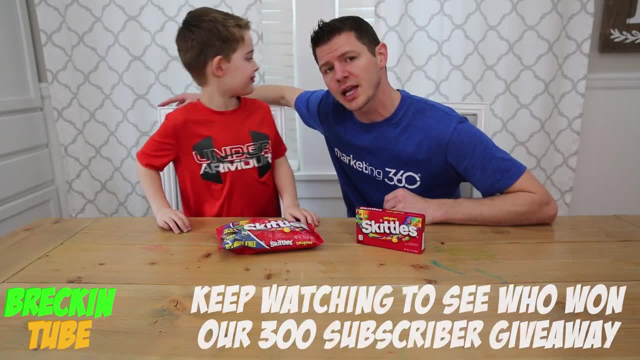 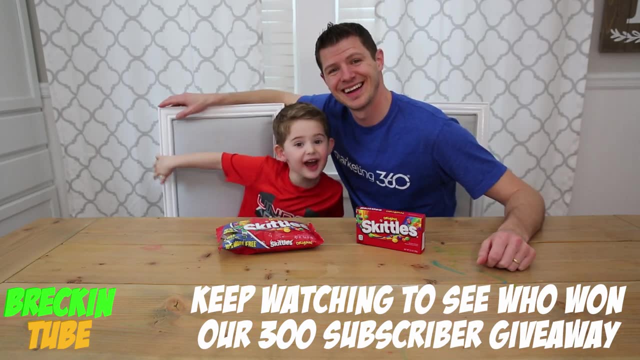 Let us know what you think about our science experiments, as well as please check out some of our other videos. Thanks for being our friends and we hope you have a great day. Thanks for being my friends. Don't forget to leave a comment. 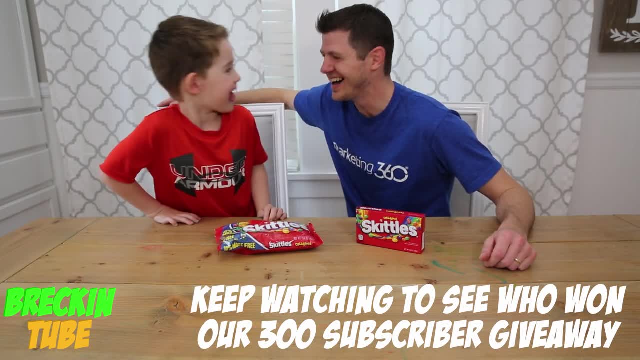 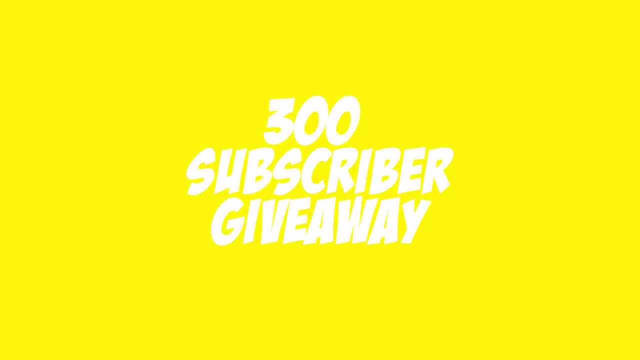 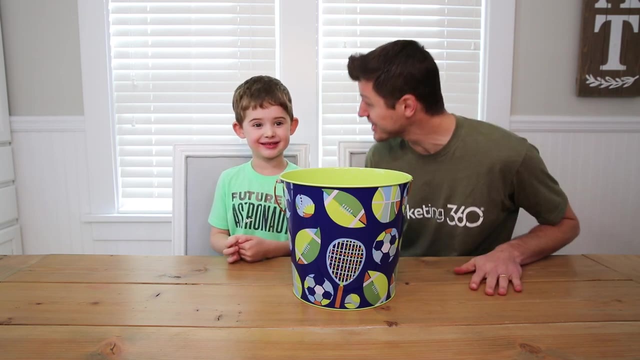 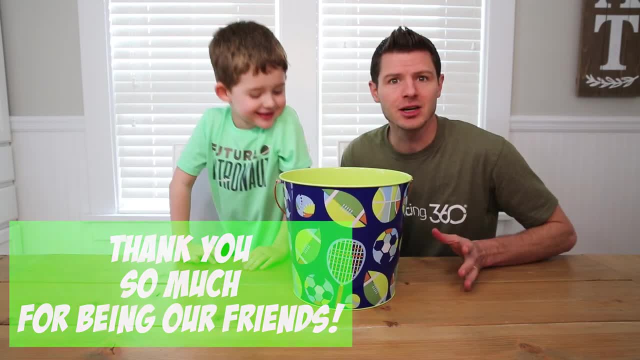 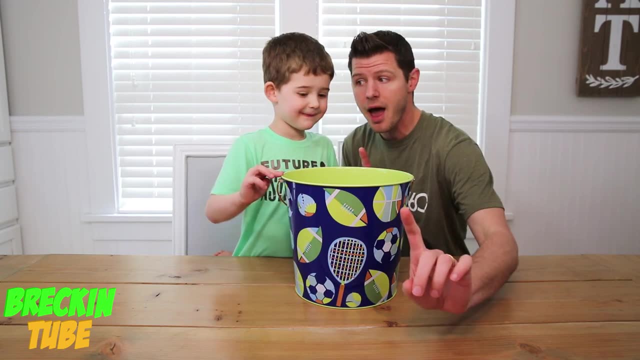 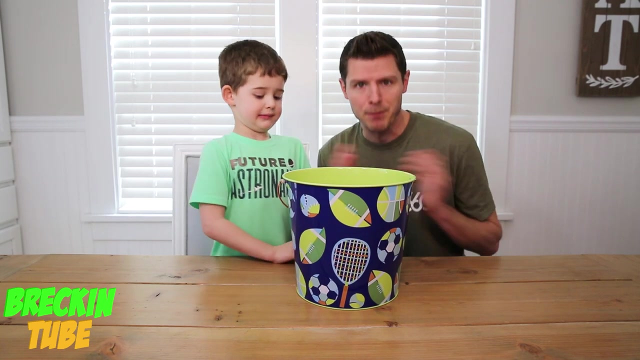 You have 300 friends already. We're giving away a Lego Ninjago Spinjitzu. So Breckin Breckin is going to choose a winner of the 300-subscriber giveaway, but we also want to say we are going to give away another secret mystery prize for our 400-subscriber. 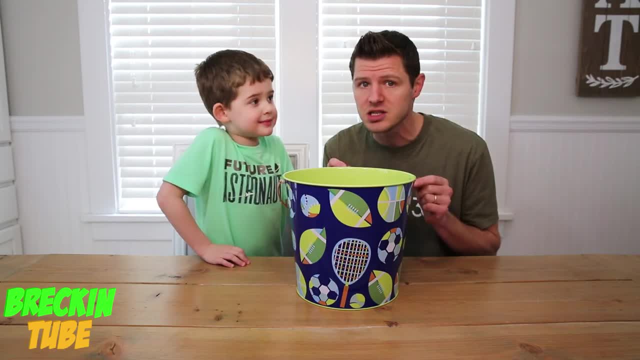 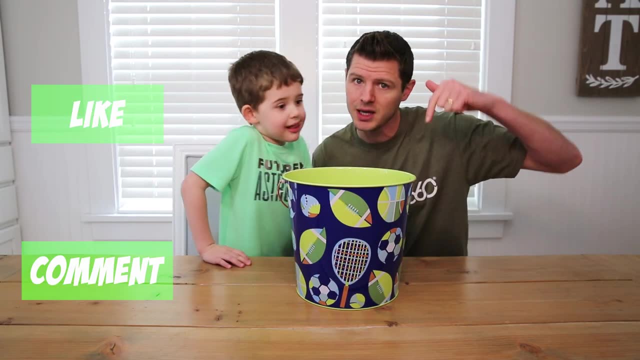 giveaway. So, in order to win, before we reveal the 300-subscriber giveaway, in order to win, in order to be entered into the 400-subscriber giveaway, like this video, leave a comment. don't forget, hit that subscribe button. 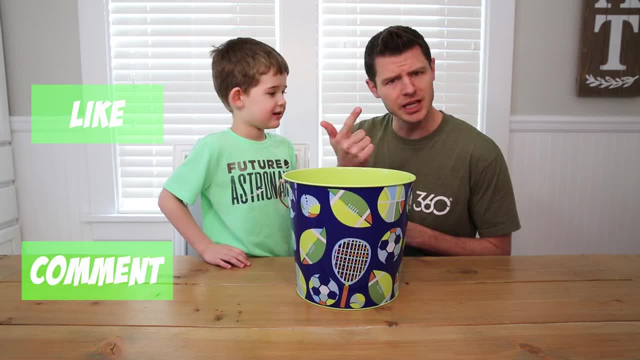 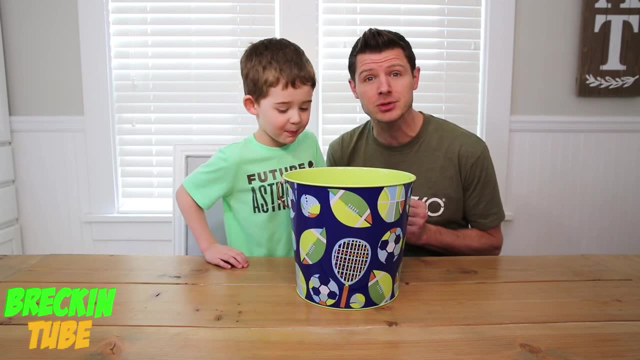 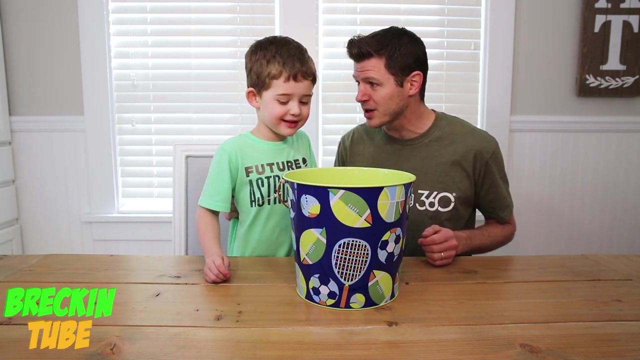 So there's three things you got to do. What is that? Like the video, leave a comment, subscribe to our channel. So you got to do all three of those to be entered into our 400-subscriber giveaway. Now, Breckin, Breckin, let's see who won our 300-subscriber giveaway. 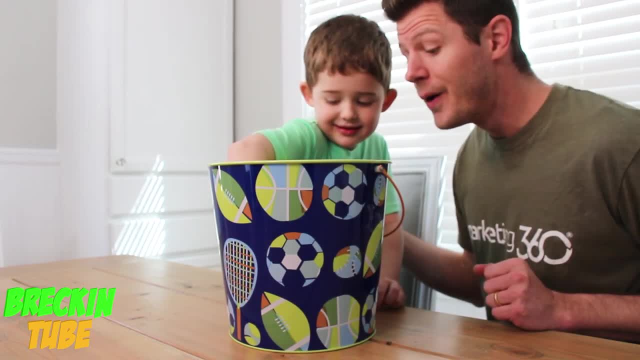 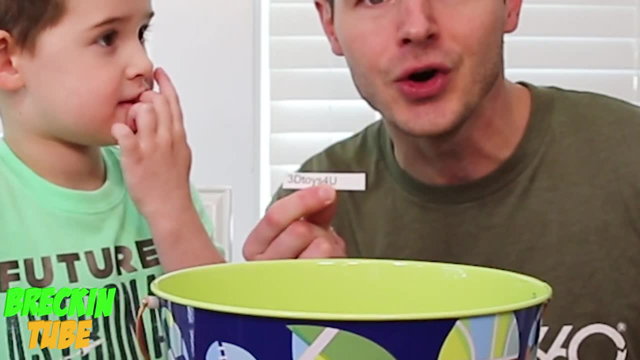 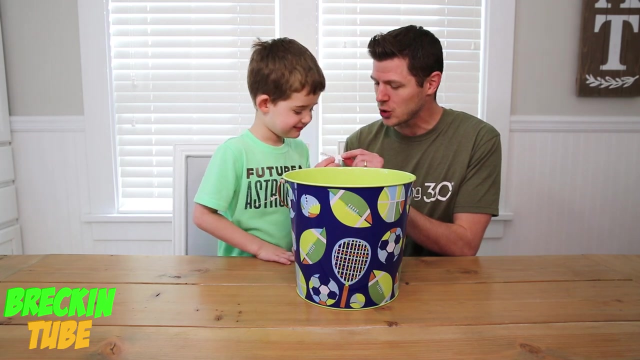 So reach on in there, Let's see who it is. Oh, let's see. This says 3D Toys For You. Congratulations, You are the winner, Congratulations, Good job. So that is so cool. So 3D Toys For You. 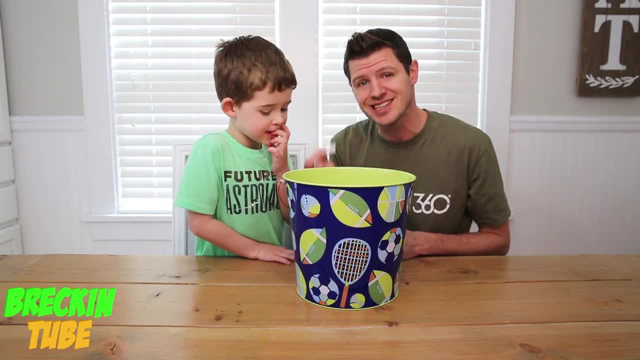 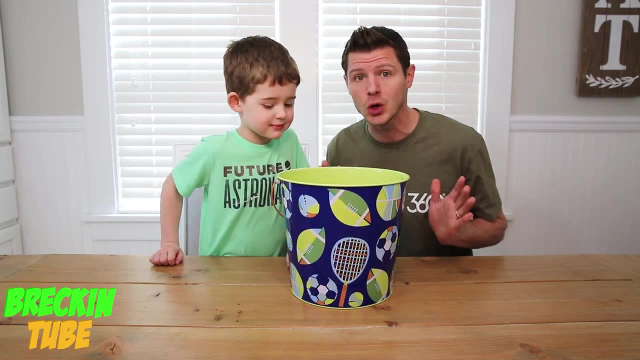 Please check your inbox in your YouTube. We're going to send you that And if you weren't the winner for today, check out. there's all those other names in there. If you weren't the winner for today, It's okay, because we love having you as a subscriber and you have a chance to win. 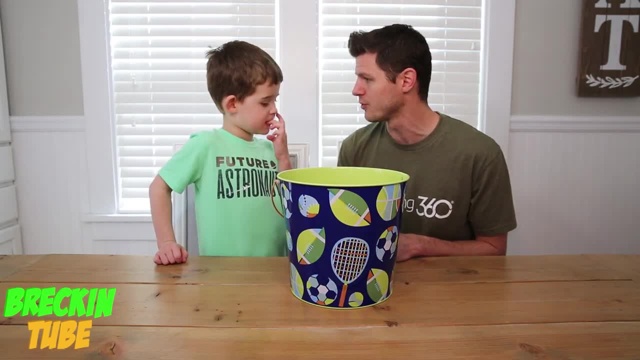 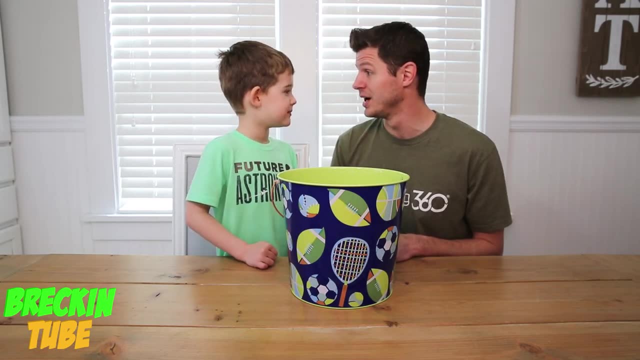 our 400-subscriber giveaway. So do you remember what they have to do for a chance to win? Uh, be picked. They have to be picked, that's right. They have to like And comment down below, That's right. 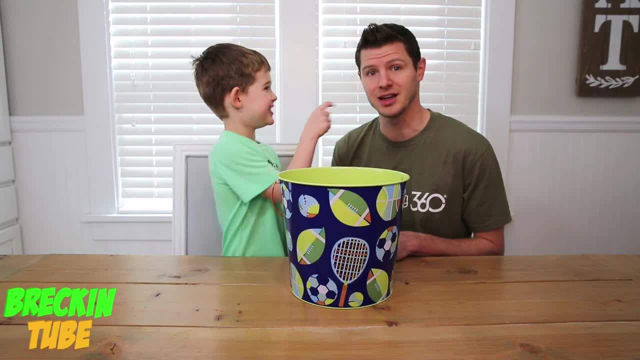 So tell them that they have to like, comment and subscribe to my channel. Tell them right there. You can tell them about them right there. Why are you pointing at me? Why are you pointing at me? I'm pointing at you.